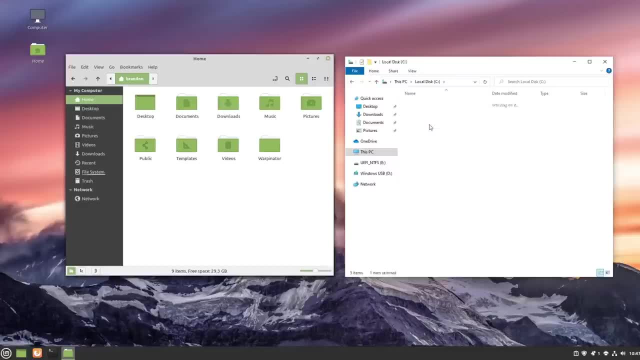 we're going to want to do is go to our local disk, go under users and then go to your actual user, and here you will see all your user directories. And now these two directories here basically serve the same function: where you can store your documents, your downloads, your pictures, your movies, all that. 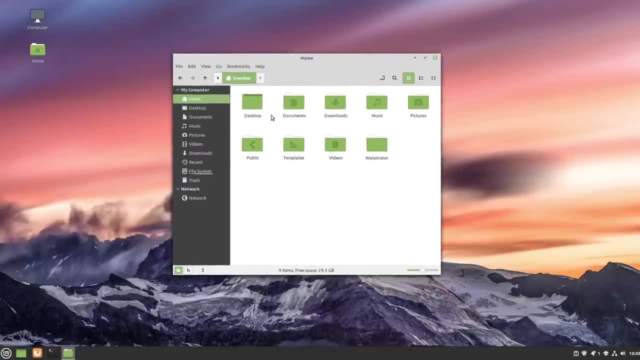 but what I want to show you real quick is how you get to this directory from your file system or from your root directory within Linux. The primary difference here from the root directory- the naming of it, is home instead of users. but then you have your username and you are in this user directory. 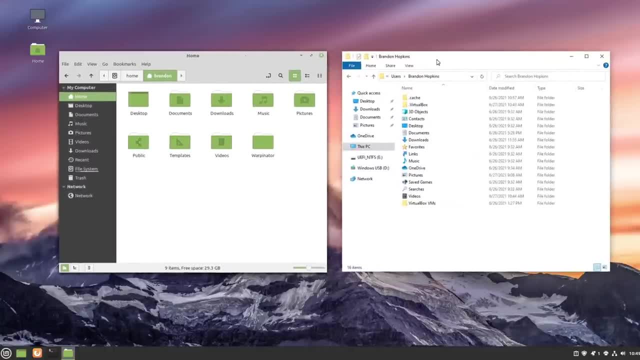 Now the similarities do kind of expand beyond this. so if I bring in my Windows file explorer here and I go to view and then show the hidden items, we're given our app data folder and here is where a lot of your actual profile local data is stored. For example, if I go over to Mozilla Firefox, you can 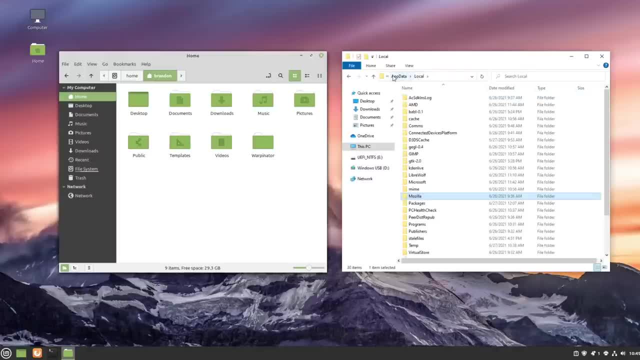 see a section for the profiles within that and there's actually a lot more. if you're familiar with, like Minecraft modding, a lot of that stuff is in here and this is the primary hidden directory within your actual user profile. Now, Linux kind of has the same thing. they're called dot files, if I. 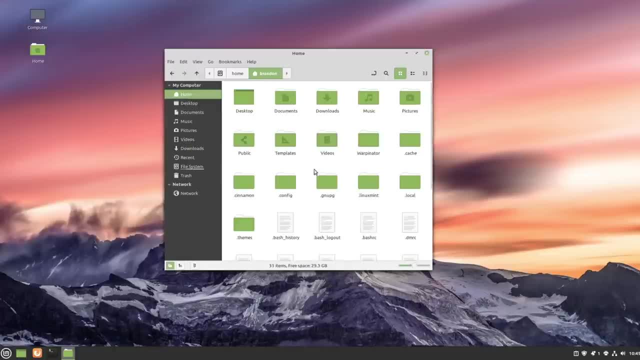 go to view and then I show the hidden files. this will give me access to those dot files And the primary purpose for these is to store your individual user configuration or specific application profiles, such as what we saw in Windows. So an example of this is either dot. 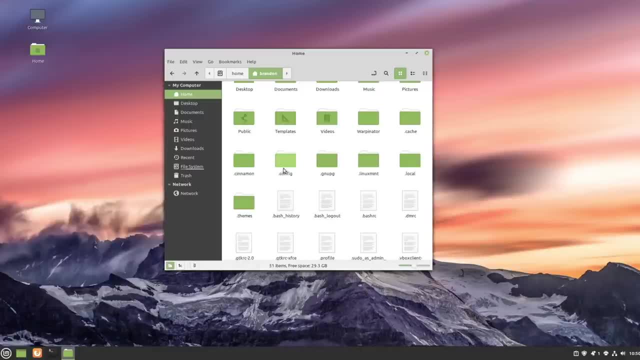 cinnamon, which will have our cinnamon configuration. we have dot config, which in here there's quite a few different things stored that we can go ahead and customize here, such as our Nemo configs, things like that. But if we go ahead and go back one that is pretty popular to go ahead and play. 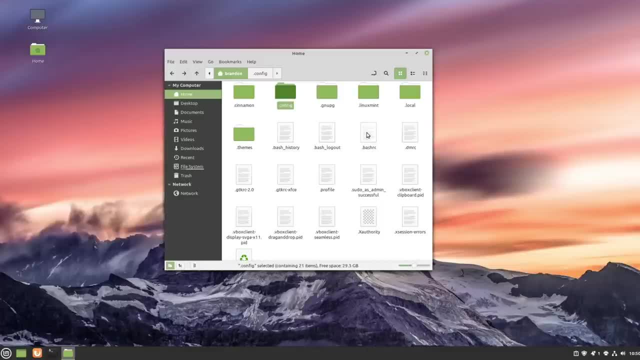 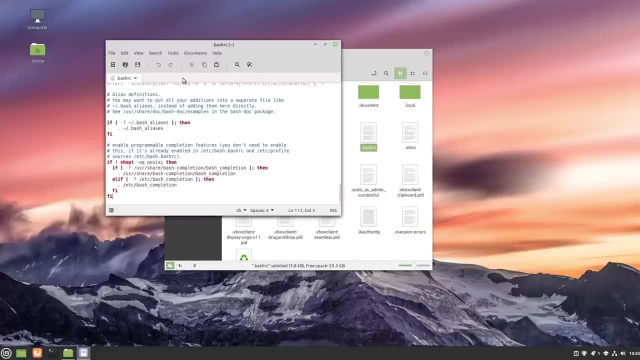 around with is your dot bash rc file. Bash rc is basically a file that you can go ahead and run on your computer. It's basically the terminal shell that you're probably running right now if you're running Linux. There are other ones, such as fish, but bash rc seems to be the most popular. 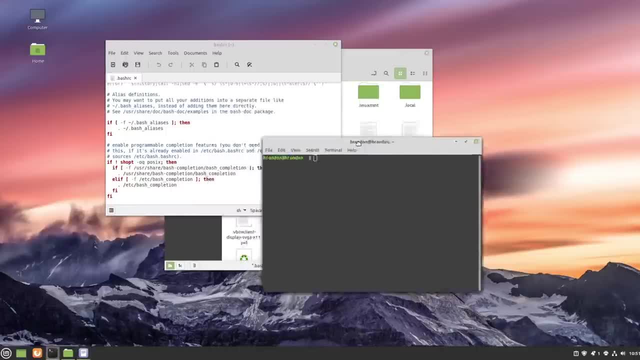 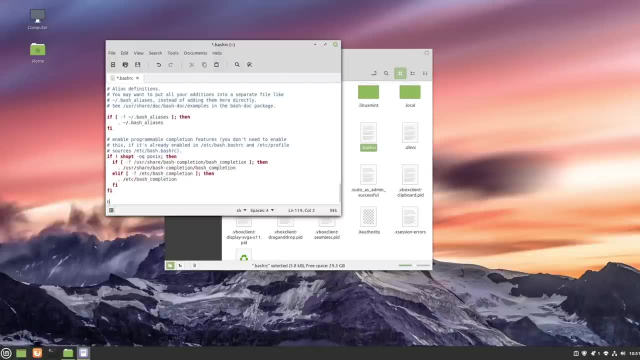 one An example of editing this configuration file. if I go ahead and open the terminal here, you can see that there is nothing special going on, but doing a simple bash rc configuration edit. we could type something in like neo fetch and then it will actually execute this command when we go. 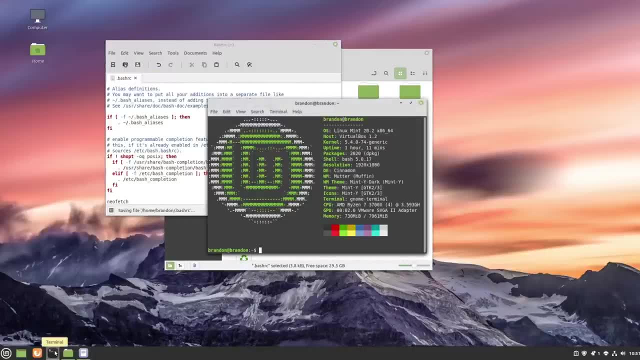 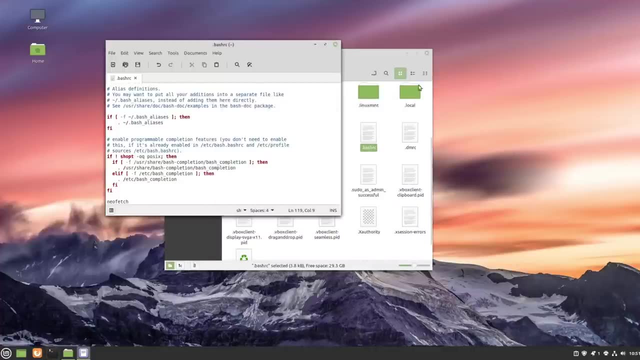 ahead and open up bash rc. So if I go ahead and save the file and they open up the terminal again and run the neo fetch program, And that's just one really simple example of a configuration edit within the Linux file system. And one thing you may have noticed is I didn't need to sudo or root. 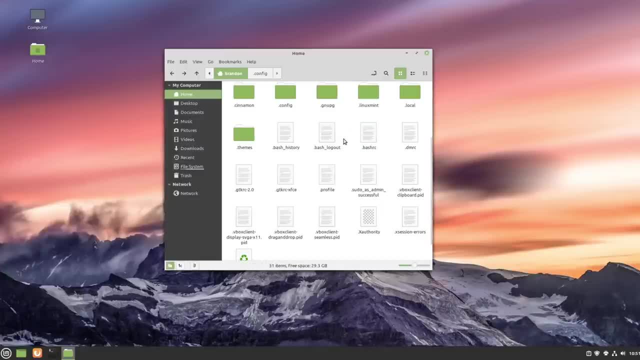 or type any passwords to go ahead and do that, because if you're working in your home user directory, you have full control over all these files and you can do whatever you want without any elevated privileges. So now what we're going to do is talk about one of the most important and 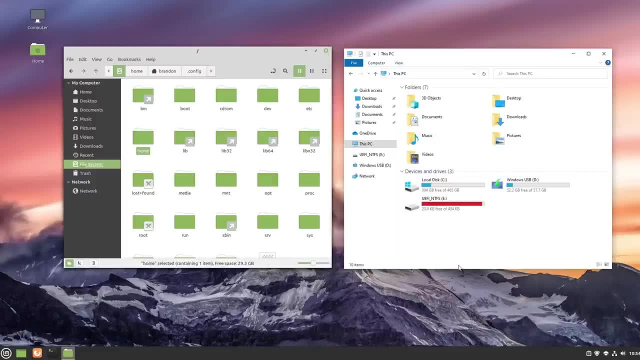 important things that you can do when you're working in your home system, And that is how your drives are connected to the file system In Windows. here you could see that all the drives are separated and they're marked by a specific letter. The C drive is your main drive, or 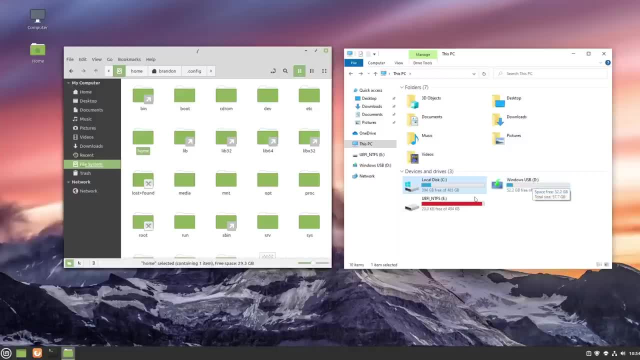 basically your root drive, And then anything else that's connected to your system is going to be given a separate letter and be separated from your main file system. This example I have here in Windows is actually a Windows USB installer with the drive D, So you can see that the root file system is completely separate from our local disk C, which is our main system. 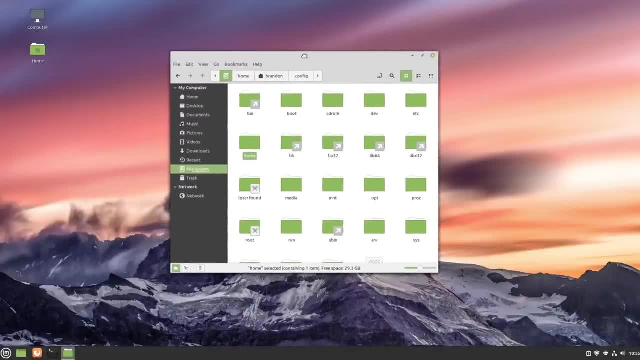 directory, While if we go ahead and look at Linux, it is working in a completely different way. Additional drives, USBs, hard drives or anything like that is actually going to be mounted within your root file system. So, instead of the separation, we see here some of the directories within this. 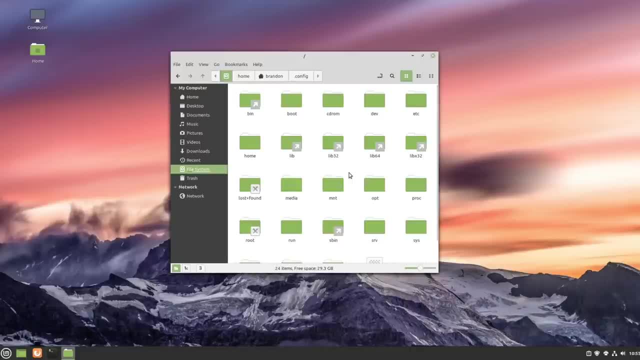 file system are actually going to be where specific drives are mounted, And the two that we're going to be looking at right now is the mount directory and the media directory. When you go ahead and plug in a USB, insert, a CD drive or whatever, it's generally going to be controlled or mounted in the 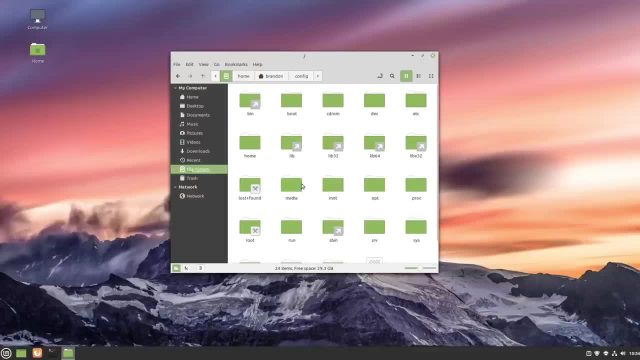 media directory right here, And the media directory is controlled by the distribution itself, While the mount directory is the user defined mounting points. A situation that you would want to define a mounting point is if you have something like a backup hard drive in your system and you wanted it to automatically mount all the time this directory. 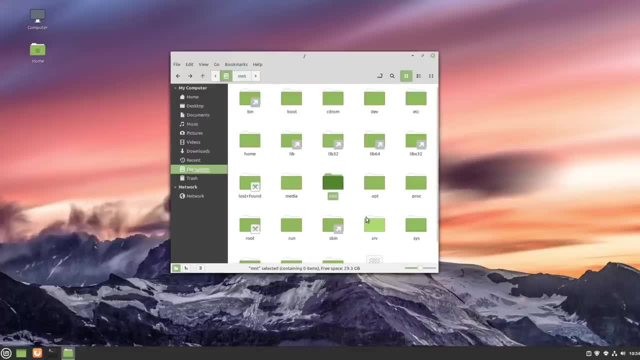 a great mounting point and you would do this by editing the fstab file or the fstab file, sorry, and I do have a separate tutorial on how to do that, and I'm going to show you an example real quick. if we go into this media mounting point and we go under my username, you can see that there is 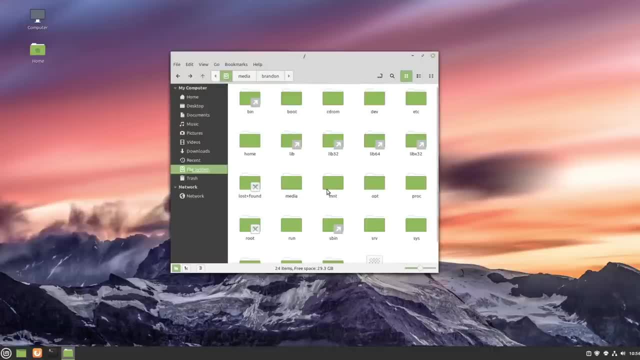 nothing here. but what I'm going to do real quick is I'm going to insert the virtual box guest additions disk, just so we can see an example of something mounting. so I went ahead and just now inserted that and we should be getting a pop-up dialog if asking us if we want to run it now. I'm 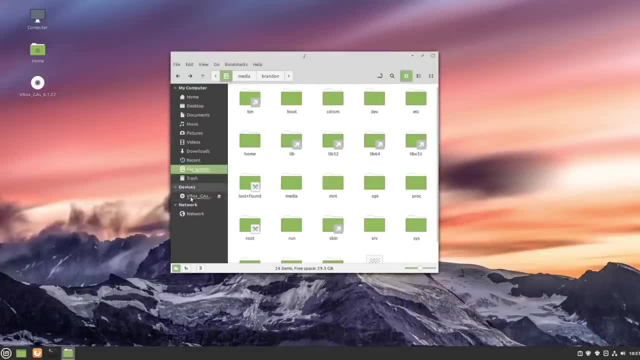 going to hit cancel for now and then right here under devices, you can see that it is separated, but this is actually just a shortcut to a directory within this root directory. so if we go over to media, which, like we said, is the one that your distribution manages, and we go to brandon, we can. 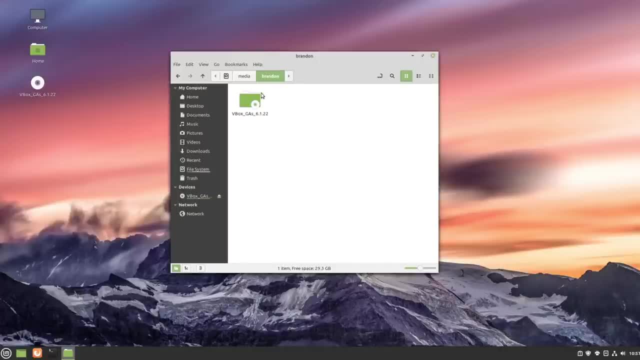 see that we have our virtual box guest addition disk directory mounted here. we open that up and we can see all of the files that we have, and then we can see that we have our virtual box guest and separate directories within that directory. So instead of having something completely separate, 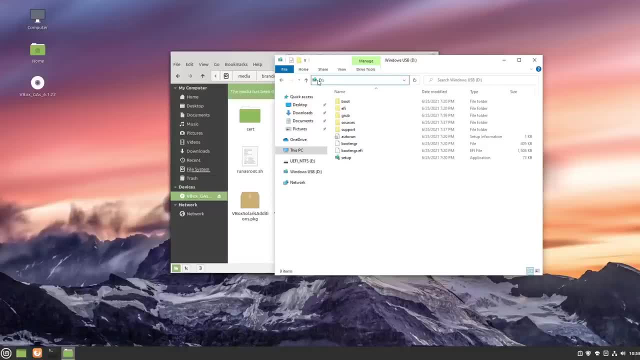 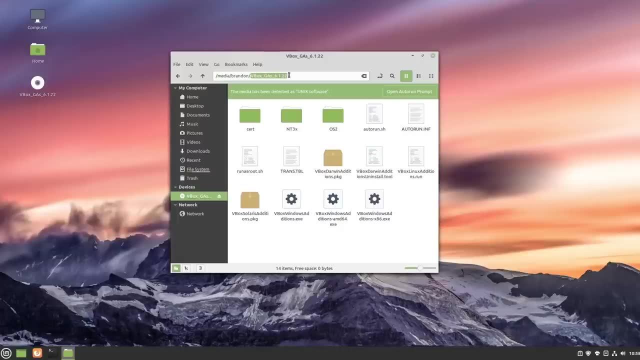 like in Windows, where if I open this up it is its own disk. right here we have something that looks a little bit like this Media Brandon, and then that drives directory. Now, my primary examples were shown in these two media and mount drives. 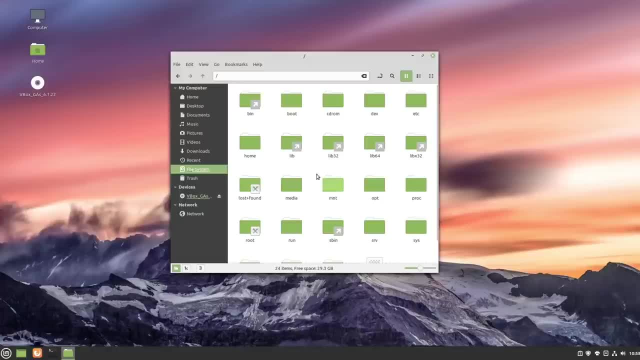 and these are generally the directories that you're gonna want to use when mounting drives. but that doesn't mean you have to use them necessarily A lot of the times, and one thing that's really cool about Linux is you can like set up your home directory. 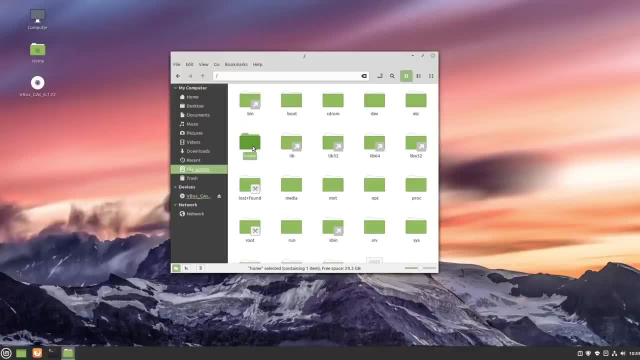 to be a completely separate drive that is mounted on your system. So if anything goes wrong with anything else or you want to change distributions or anything like that, this could be a completely separate drive. So your entire user profile, all your dot files. 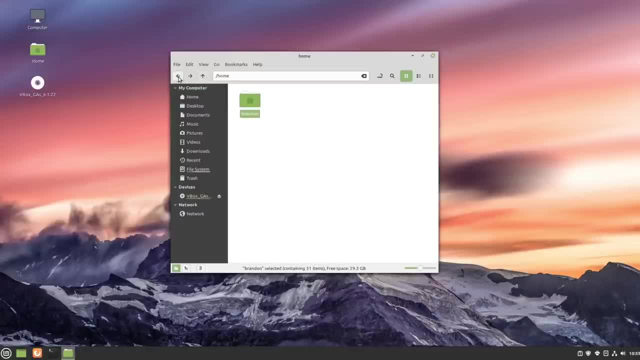 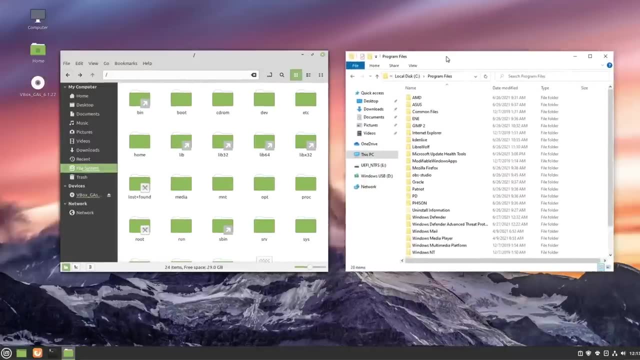 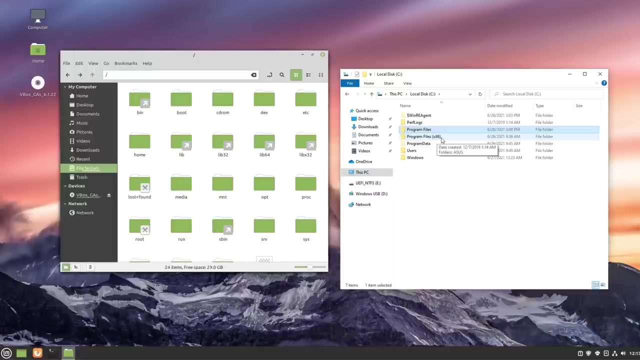 and all your important documents or whatever, are on a completely separate drive than the drive that your Linux distribution is actually installed on. All right, so next we're gonna go ahead and talk about program files. Now, in Windows we have program files and program files x86, depending on the architecture. 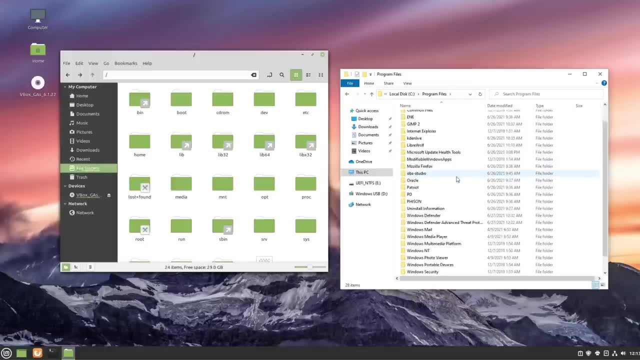 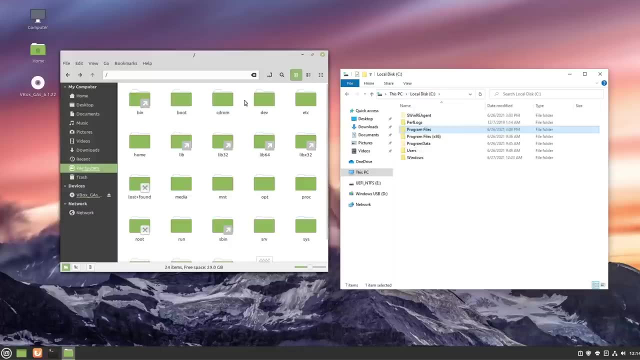 that the programs were written for, And in these program file folders we can see both system-wide and user-installed programs. Now there's actually some pretty decent equivalencies within the Linux Unix file system here, and that's gonna be in two folders. 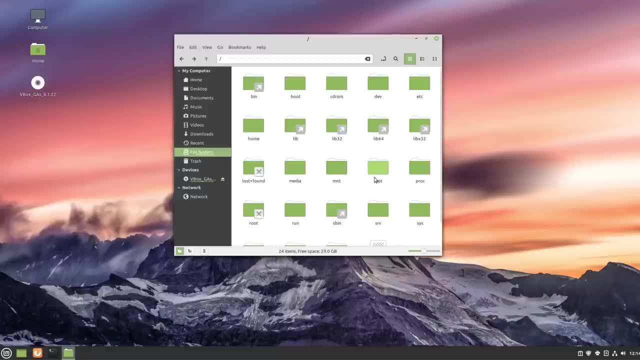 So let's go ahead and take a look at those. The first one is gonna be this opt folder. Now, this is gonna be the program files or the applications and software that the user actually went ahead and installed. So on this system, the only things I've manually installed- 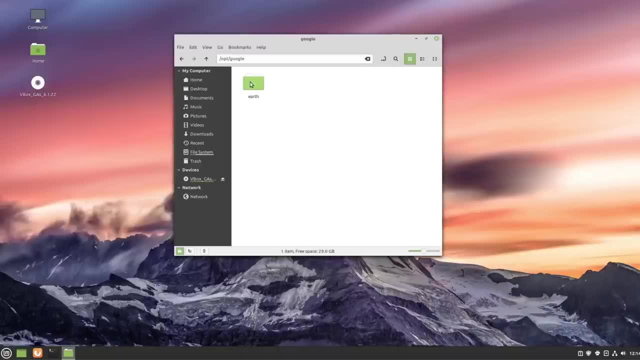 is the VBox Guest Edition drivers and Google Maps. So you can see Google Earth Pro And here are all those program files to make it so that the Google Earth application can run And it kinda looks the same in Windows if we go into program files. 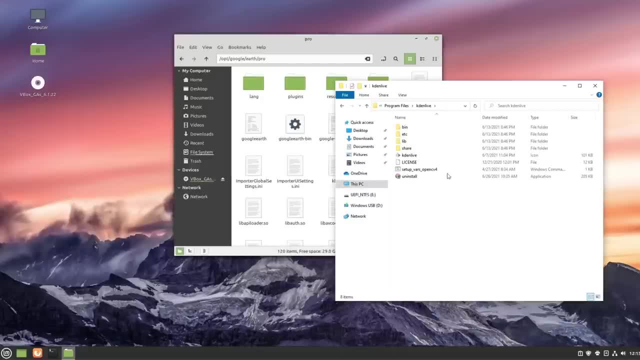 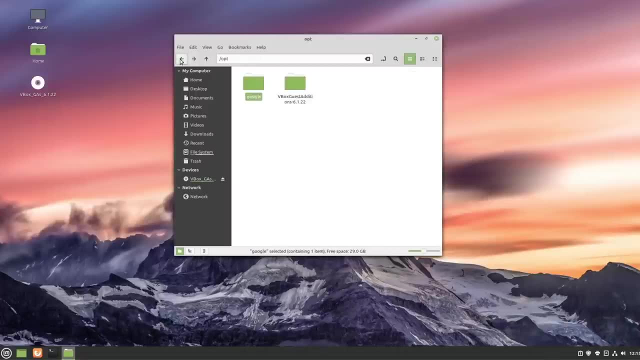 and open up a random application such as Kdenlive. These are those specific program files. Now, additionally, there's another folder that we can go ahead and take a look at, and that is gonna be either bin or sbin, And what these are are folders or directories. 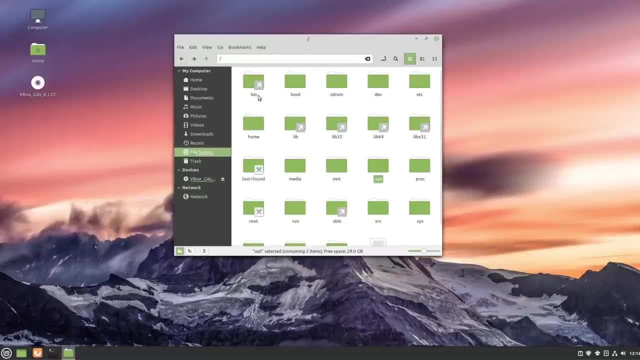 that contain various binaries for programs that are installed by default in your system. Sbin means system bin, I'm pretty sure, And bin is just bin. Now in here you can see applications. A lot of them are applications you're gonna want to run from the terminal. 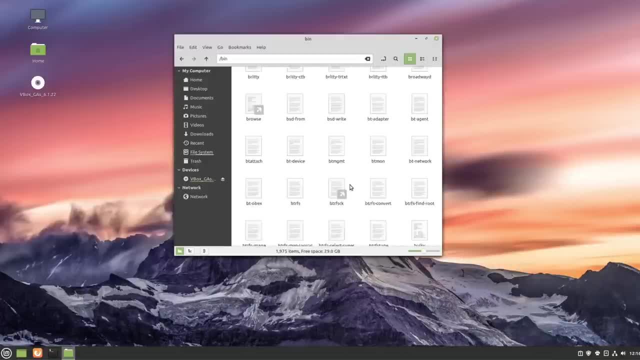 apt-get, and there's others, such as MV cat C-A-T. So if I go over to the Cs we can see cat is in here. And there's others, such as the directory, modifying commands such as move, remove, copy paste, things like that. 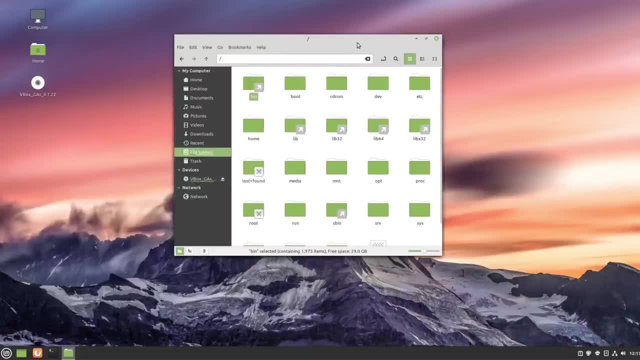 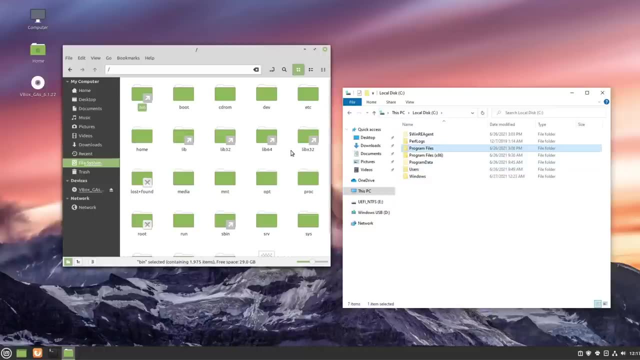 So overall, those are the program files equivalencies in Linux. Now, from here on out, it gets much more difficult to kinda match up various equivalencies between the different file systems, because all we really have left here is Windows. In Windows, this is your operating system. 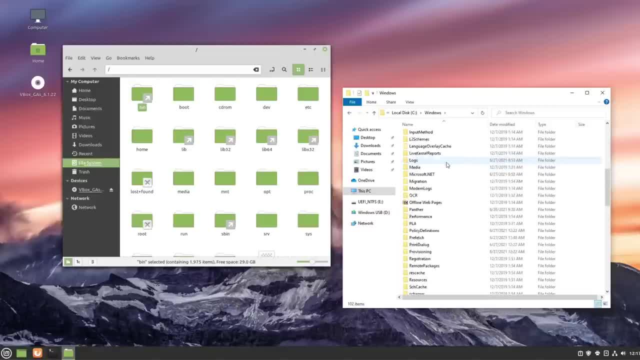 But even with that said, there are some equivalencies we could kinda match up here, And the most obvious one is boot. So in this boot directory are the files and configuration that are required to make Windows go ahead and boot up, And we kinda have the same thing going on over here. 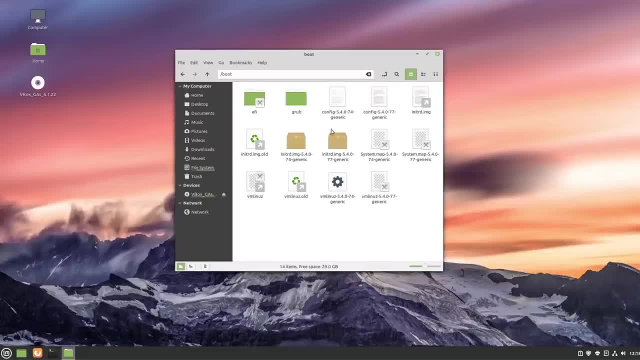 in the boot directory. This is where all of our grub stuff is stored, including the essential files, configurations, well, system-wide configurations, and things like that. So this is where all of our grub stuff is stored, including the essential files. 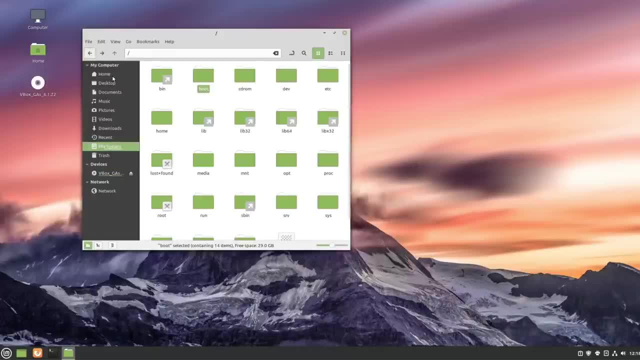 configurations and things like that. Now for another equivalency, and I am gonna be kinda stretching here a little bit, but that is these lib folders here. These are your libraries. So these are helpful libraries that are used by the system and the best thing I could compare them to. 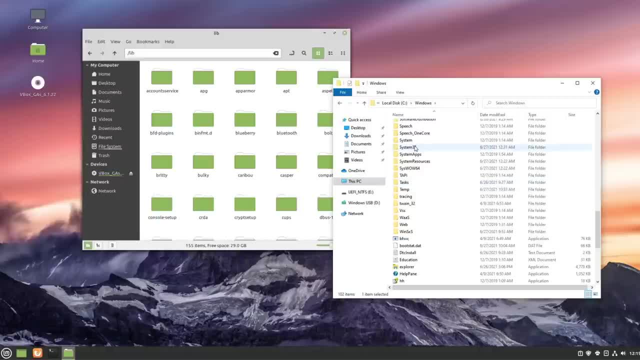 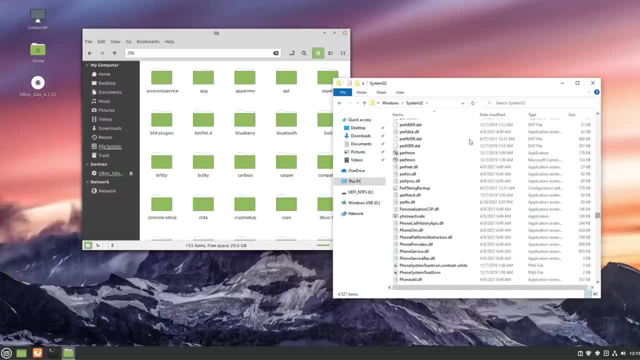 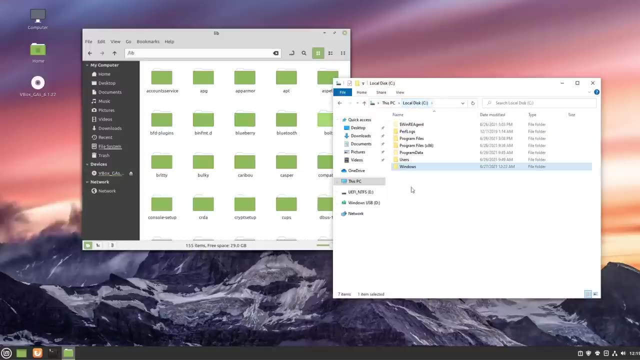 is if I go into the trustee system 32 folder. these are all the DLL files that basically make Windows run and these are kinda the equivalent to these library files. here And after those. it's really hard to come up with equivalencies and comparing to the Windows file structure. 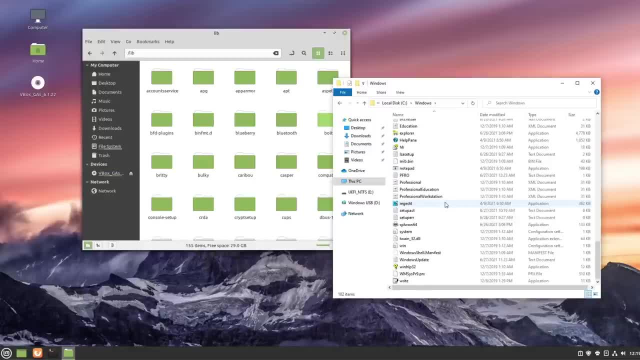 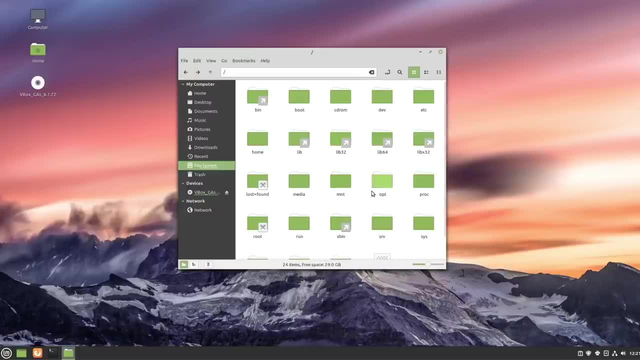 in the actual Windows directory, because everything's really spread out. So the only thing I can really do going forward is kind of explain what some of these directories are very briefly, because it's kinda hard to match up Windows equivalents at this point, And we'll start up with CD-ROM right here. 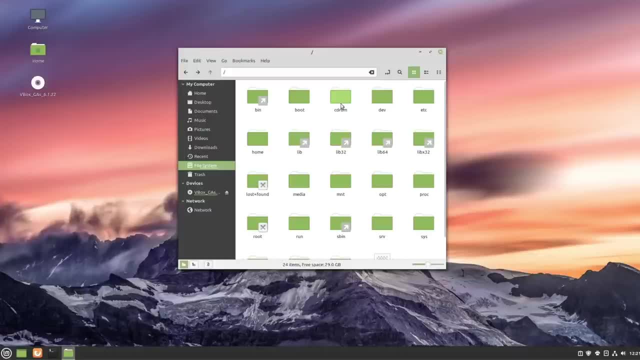 Like we explained earlier with mount points, this is another mount point that's not really used anymore, but it's kinda just left there for compatibility. So it's not really used anymore, but it's kinda still there for compatibility reasons. And right here we have dev. 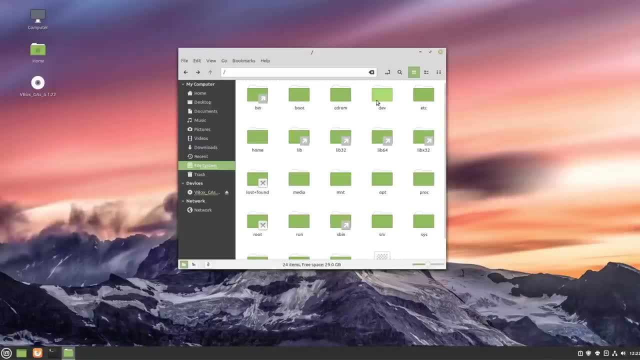 and what this is is your hardware: disks, webcams, things like that. Whatever hardware in your system that's plugged in is gonna be recognized in here as a file. And this goes all the way down to something like: if we go over to the Ss, the SDA- 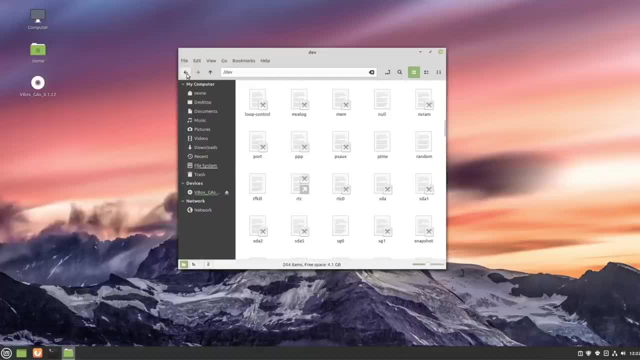 even separate partitions have specific files in here that kinda link to those devices. The etc folder or etc is gonna be your system-wide configuration files. It's gonna be playing around in here a little bit, but to edit anything in here you're gonna want to do that as a super user. 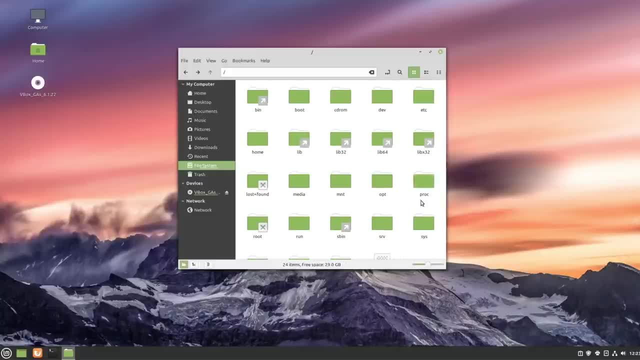 And from here we've talked about all of these up till process or the PROC folder, and this is where it's gonna contain a lot of your system information. So if I go ahead and open that up and scroll down to the bottom, for example, 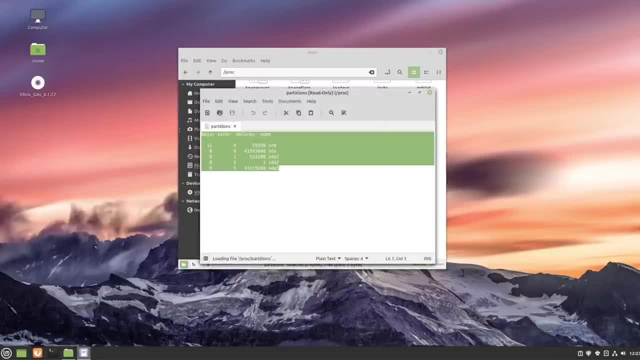 I can find things such as partitions. open up this file and I can see some information on various partitions in my system. If I scroll up a little bit more, I can find CPU info here and then get information on the CPU that's in my system.